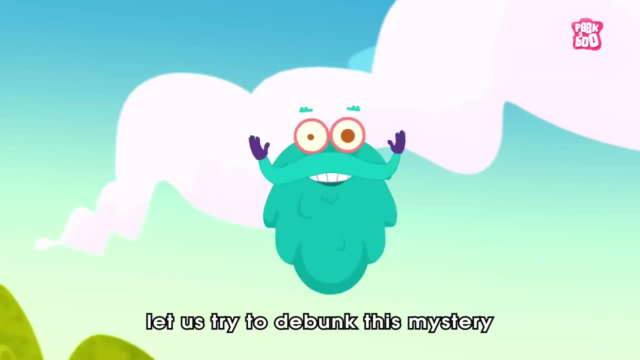 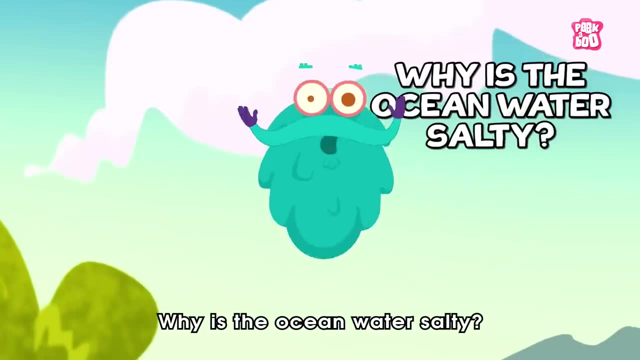 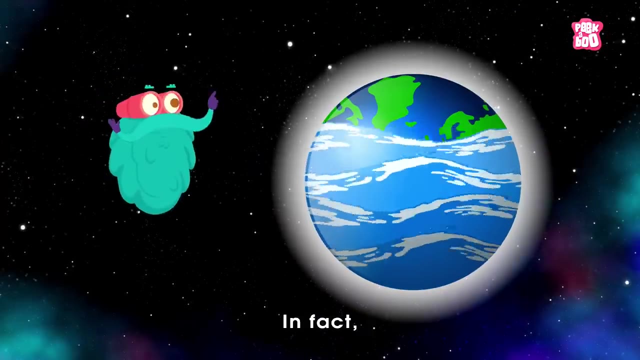 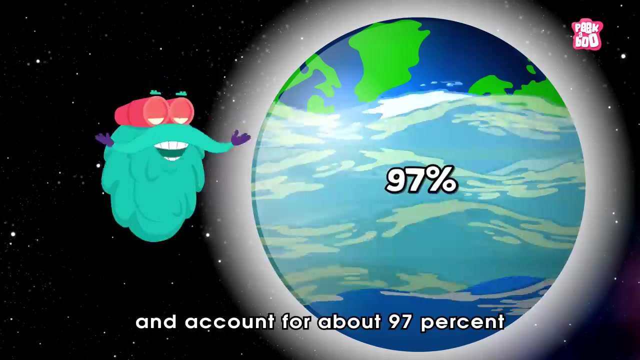 Well, in today's episode, let us try to debunk this mystery and answer a deep question: Why is the ocean water salty? Zoom in The world is surrounded by water. In fact, oceans cover 70% of Earth's surface and account for about 97% of all water. 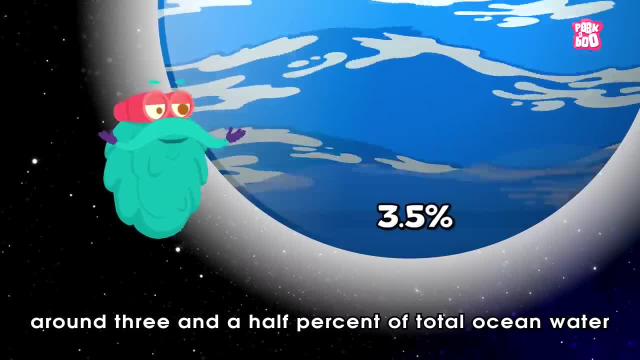 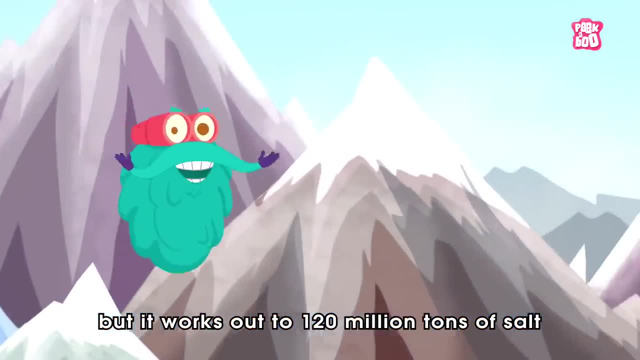 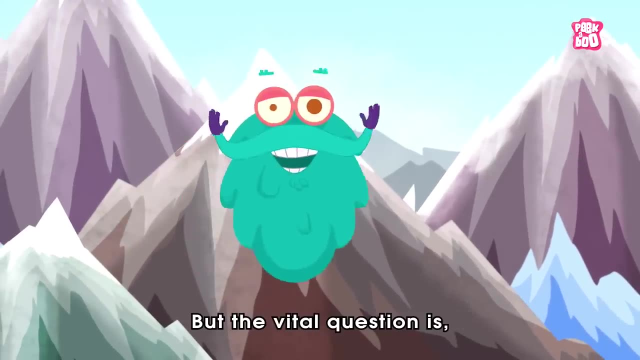 And approximately around 3.5% of total ocean water is salt, Which may not sound like too much, but it works out to 120 million tonnes of salt per cubic mile of sea water. But the vital question is: where did all the salts come from? 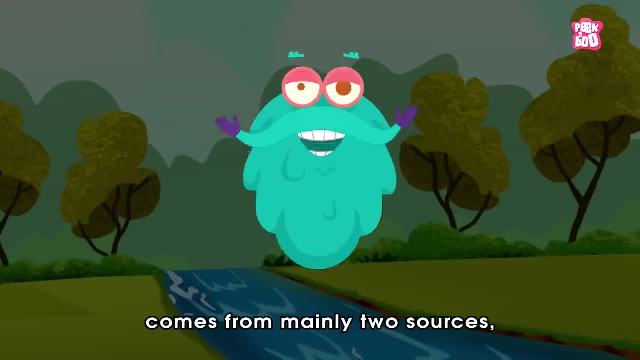 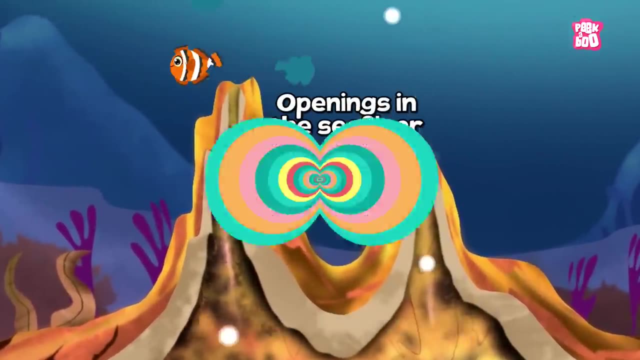 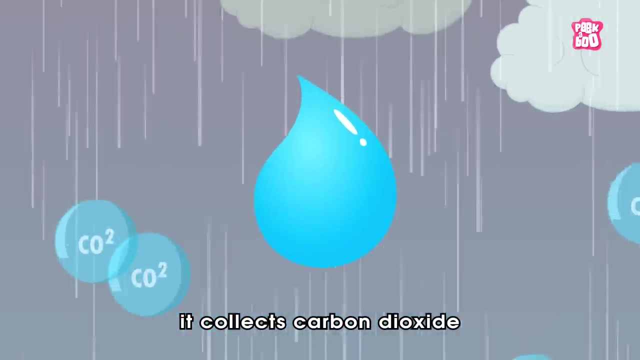 Well, salt in the ocean comes from mainly two sources: Runoff from the land and openings in the sea floor. You see, when the rain forms and pours through the air, it collects carbon dioxide from the atmosphere on its way, turning the fresh water slightly acidic in nature. 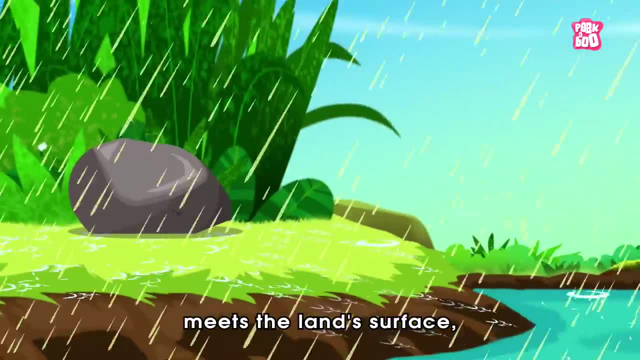 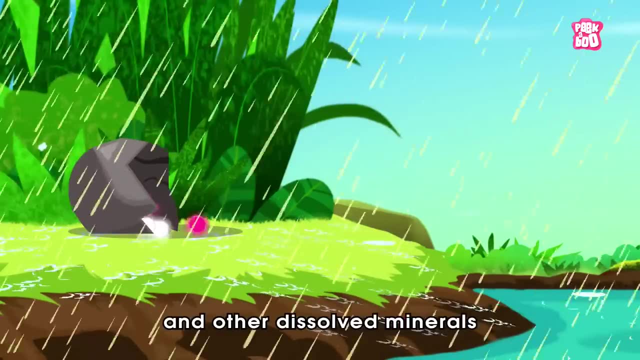 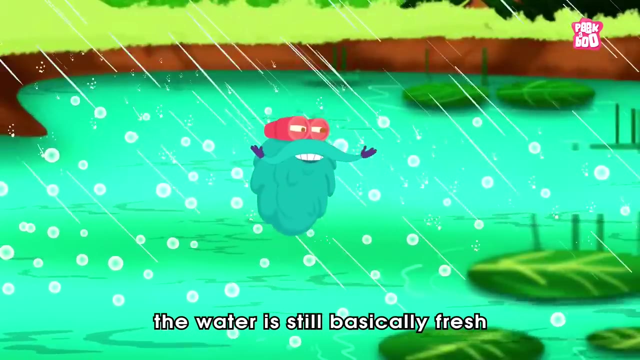 And once this acidic water meets the land surface, it erodes the rocks and picks up small amounts of salt and other dissolved minerals already present in the rocks. At this point the water is still basically fresh. There is some salt in it, but usually not enough to make it undrinkable. 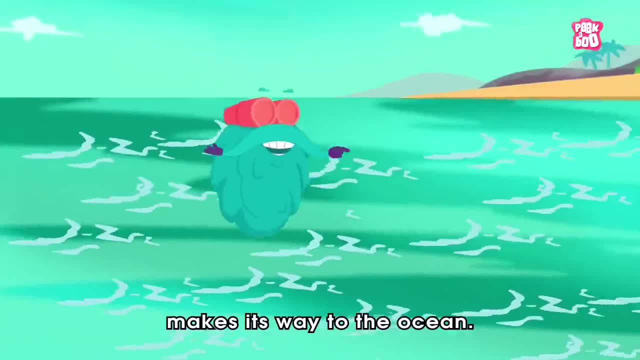 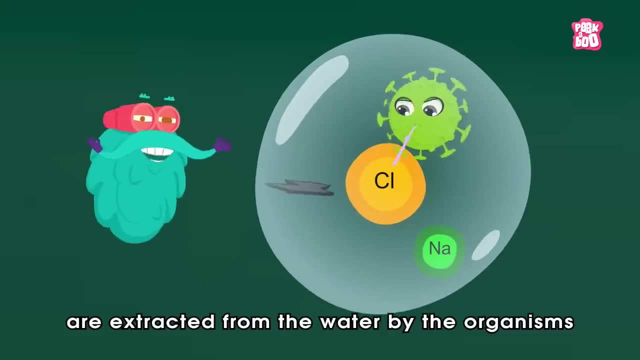 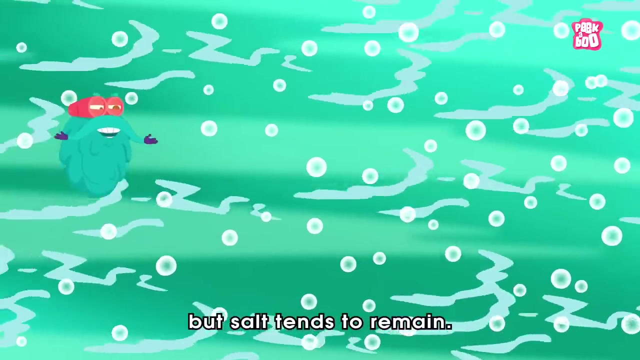 But when this mixed rainwater makes its way to the ocean over there, some of the dissolved minerals, such as calcium, are extracted from the water by the organisms through a biological process, But salt tends to remain, thus making the water undrinkable and salty. 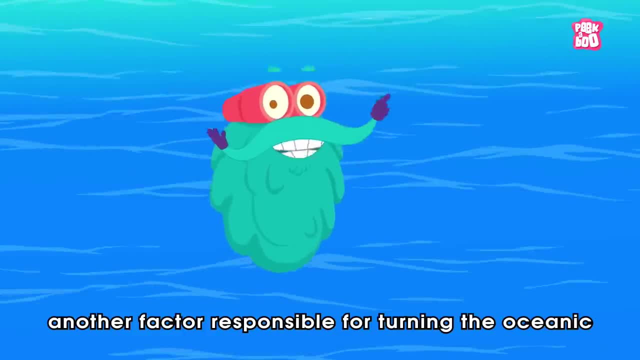 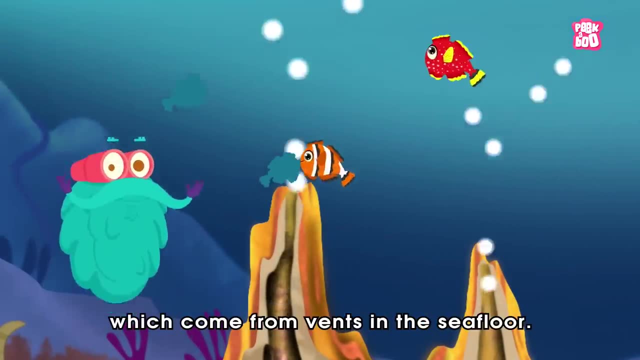 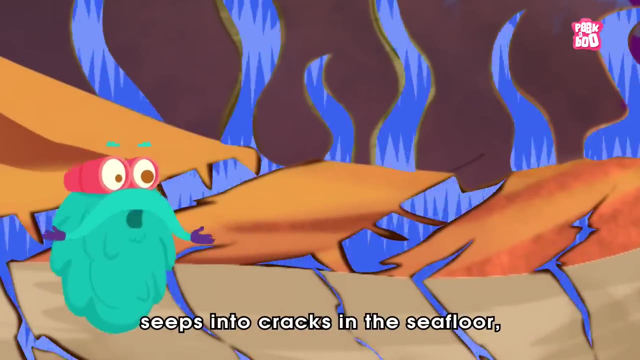 But not only that. another factor responsible for turning the oceanic water salty is hydrothermal fluids, which come from vents in the sea floor. You see, when the salted ocean water seeps into cracks in the sea floor over there, it gets heated by magma from the Earth's core.